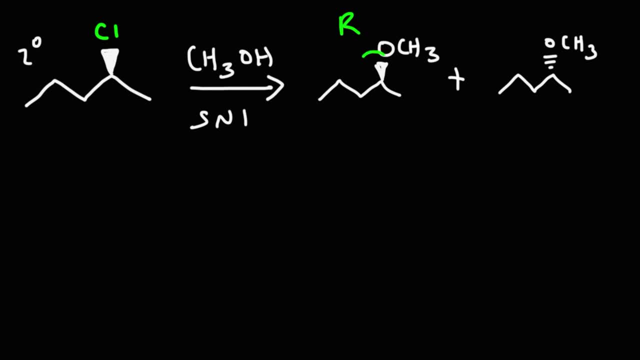 So this is the retention product, because we could see that it retained the stereochemistry at the chiral center, and this is the inverted product. So here the configuration at the chiral center is S. It's S here as well, but here it's R. 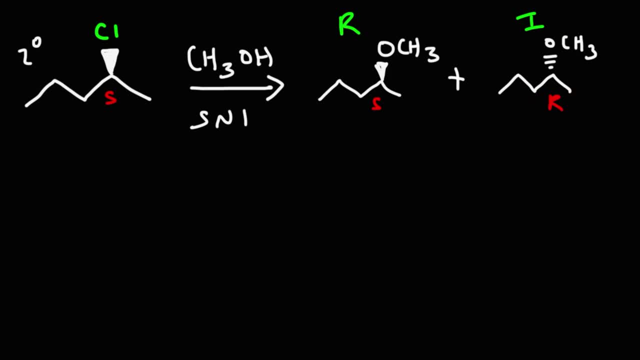 So that's why this is the inverted product. Now, in an SN1 reaction we typically don't get an equal amount of the retention product and the inverted product. We get an unequal racemic mixture. So the retention product, we might get 40% of it and the inverted product, we might get 60%. 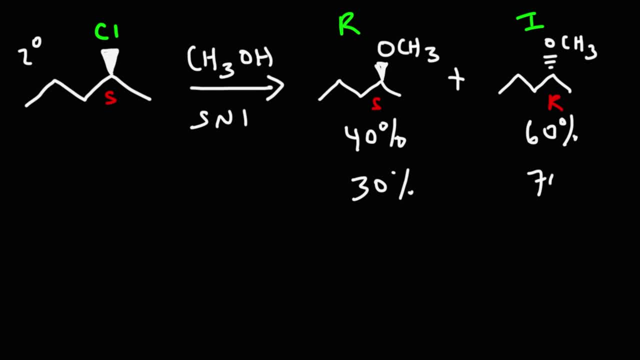 In some cases it may be 30-70 instead of 40-60. But nevertheless we do observe that it's an unequal racemic mixture. We get more of the inverted product than the retention product. But the question is why. 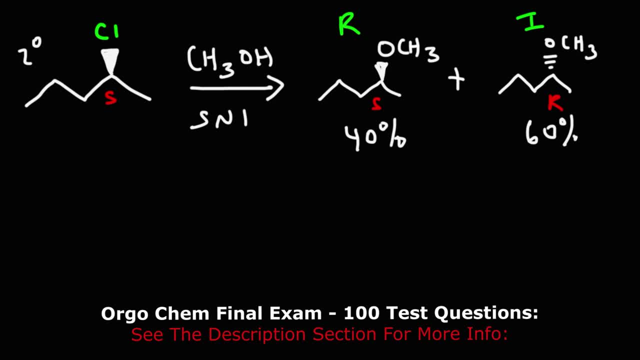 Why? Why do we get more of the inverted product than the retention product? The answer has to do with something called the intimate ion pair. Now let's talk about the mechanism for this reaction. In the first step, the leaving group is going to leave. 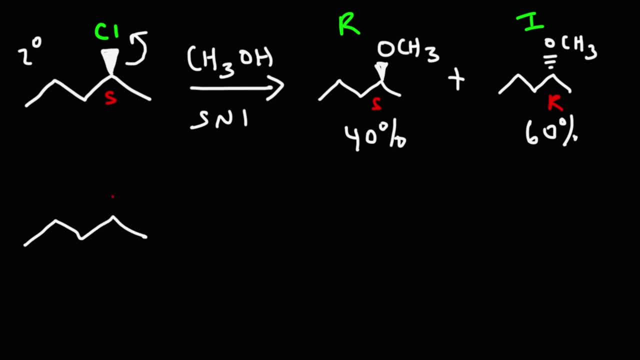 And we're going to get a carbocation, a carbon with a positive charge. Now, when the leaving group leaves, usually it's not very far away from the reaction. So we're going to get a carbon with a positive charge And we're going to get a chloride with a positive charge. 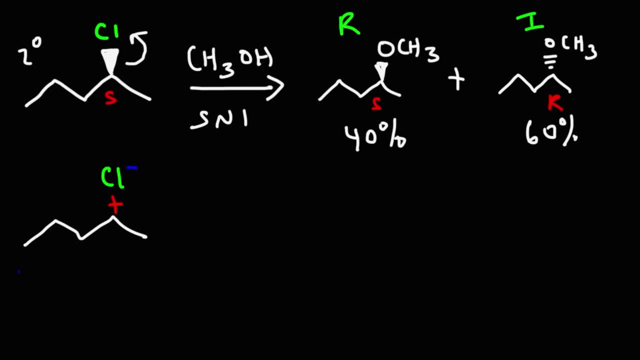 We're going to get a chloride with a negative charge And we're going to get a chloride with a negative charge. So even though they've broken apart, the chloride is likely relatively close to the carbocation. Now the solvent methanol could solve a chloride and move it away from the carbocation. 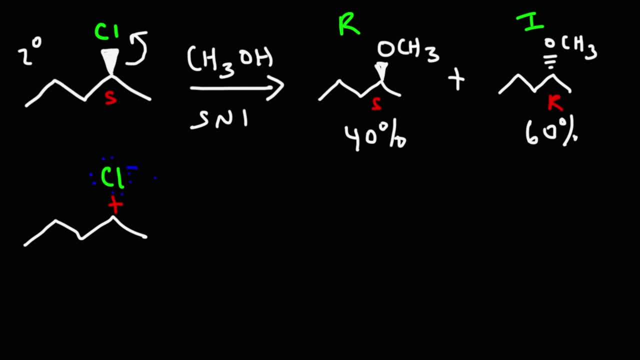 But a lot of times they're pretty close And in this situation, when these two oppositely charged ions are close to each other, that's what is known as The intimate ion pair Keyword. intimate- that means they're very close to each other. 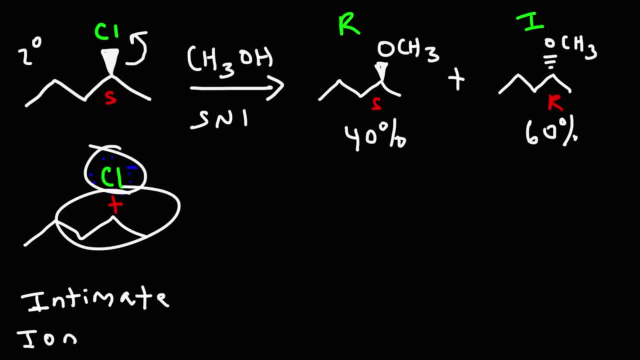 And we also have a pair of ions. This is one ion, that's two. two makes a pair, So that is the intimate ion pair. Now methanol, which is the solvent, is going to behave as a nucleophile, So this is going to be a solvolysis reaction. 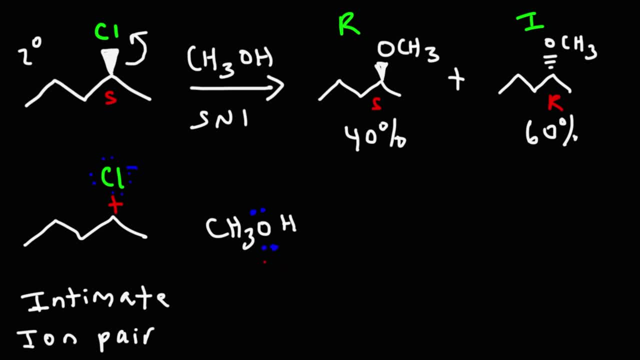 The solvent could approach the carbocation from the back, which will give us the inverted product, Or it could try to get to the carbocation from the front, which will give us the retention product. In this situation, is it easier for the nucleophile to approach the carbocation from the front or from the back? 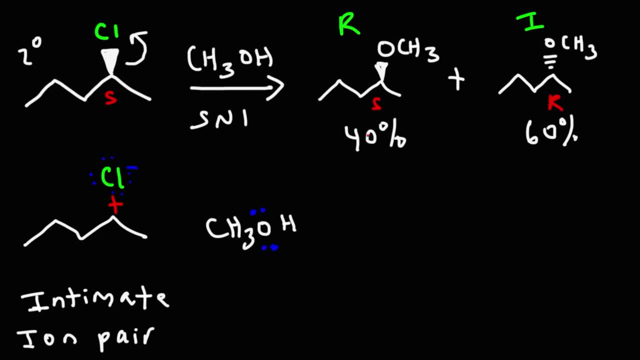 What would you say If it tries to approach from the front? notice that it's going to be repelled by the chloride. The chloride ion has a negative charge And the oxygen of methanol, which is the nucleophilic part of methanol, that has a partial negative charge. 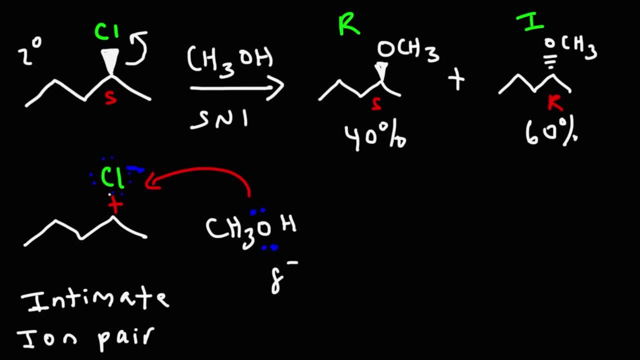 So those two are going to repel. So it's going to be harder for methanol to approach from the front. If it approached the carbocation from the back, there's no problem with that because the chloride is not in the way, And that's why we get more of the inverted product than the retention product. 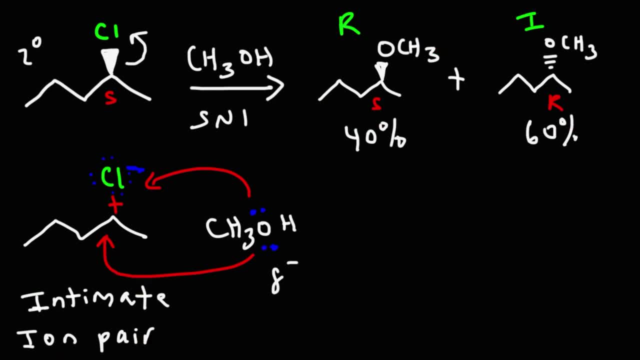 It's because of the intimate ion pair. The nucleophile can easily approach from the back because the chloride ion is not in its way, But as it tries to approach from the front, it's going to be repelled by the chloride ion, giving us less of the retention product and more of the inverted product. 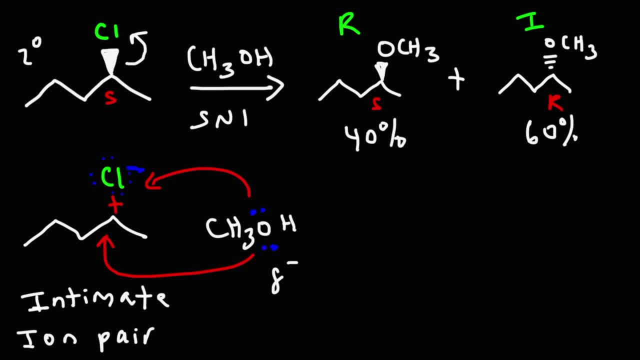 So that's the basic idea behind the intimate ion pair. Now if we, If we were to slow down the reaction and allow more time for the chloride to be fully dissociated into the solvent, let's say if the solvent, if the chloride were to move away in the solution? 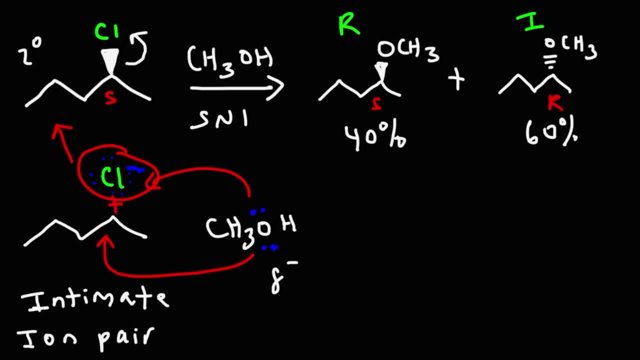 then methanol would be free to attack from either side And we would get closer to a 50-50 mixture as opposed to a 30-70 or 40-60 mixture. But it all depends on the proximity of the chloride to the carbocation. 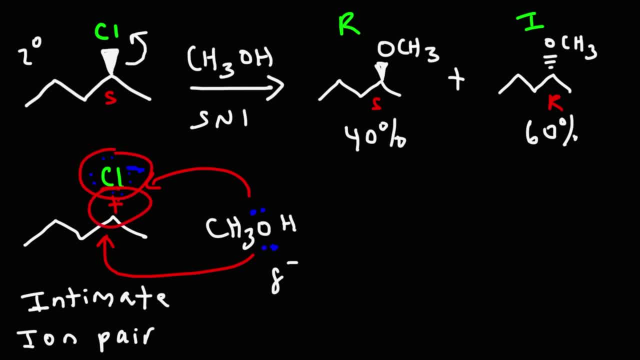 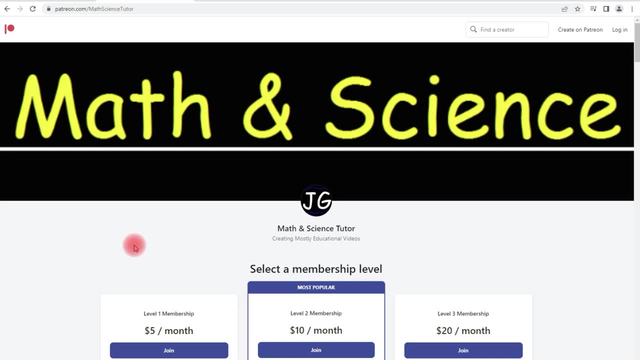 Okay. So the closer these two are, the more likely we're going to get an unequal racemic mixture. Now, for those of you who are interested in downloading that practice test, here's how you can do it. So if you go to patreoncom slash math science tutor, it'll take you to my Patreon membership page.